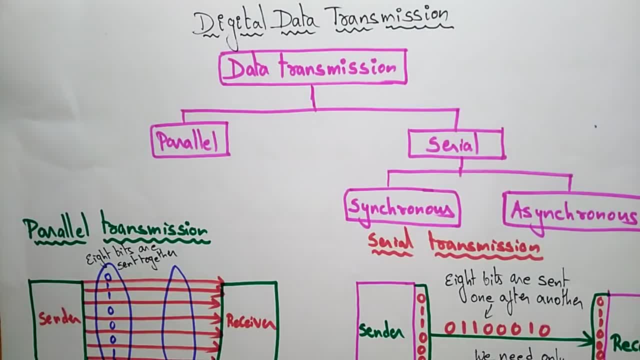 Hi students, welcome back. Coming to the next topic, that was a digital data transmission. So we already know the data transmission, So the data transmission that can be using digitally, how the digital data is going to be transmitted. So, before going to the topic in depth about the digital data transmission, let's see the overview of data transmission. 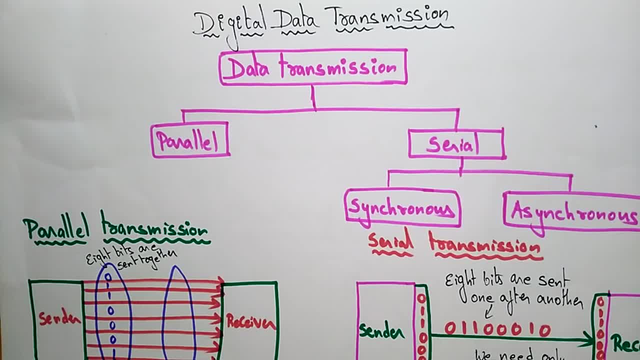 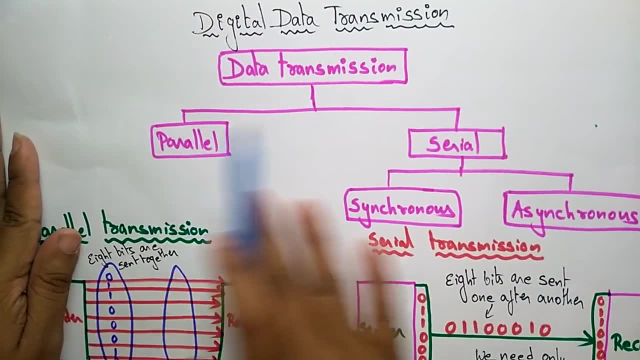 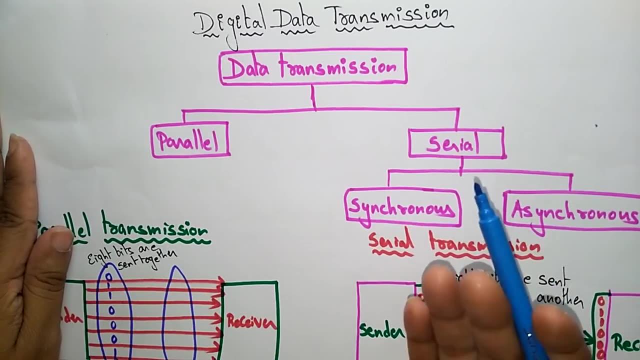 So you already seen in the different concepts in the whatever the videos I explained in the computer networks. There you can see the data transmission is of two types. One is the parallel and the serial. If you want to send the data from sender to receiver, the data communication, that data can be transmitted over a physical media, in parallel or in serial. 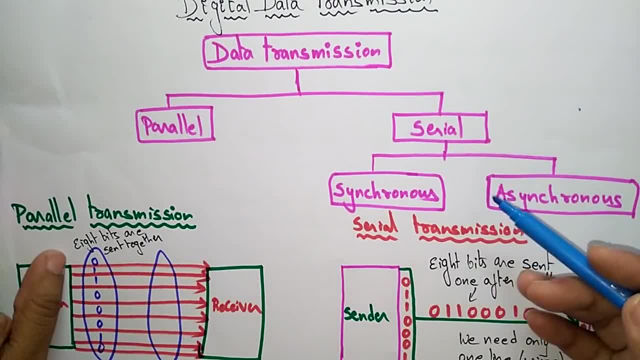 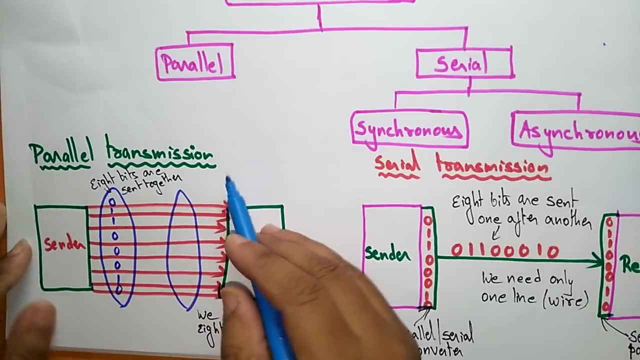 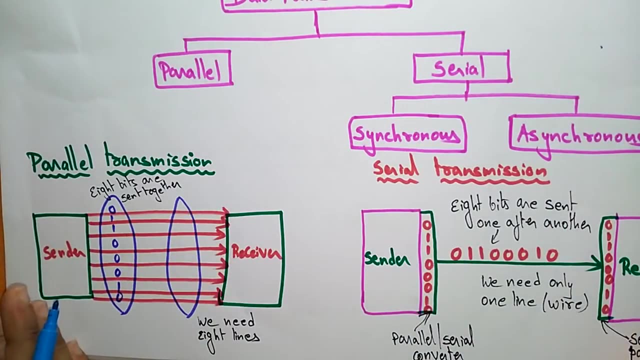 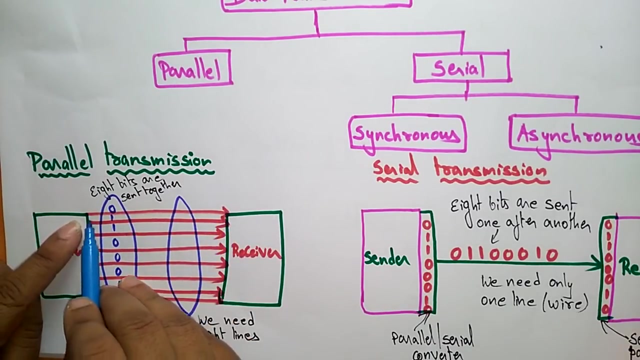 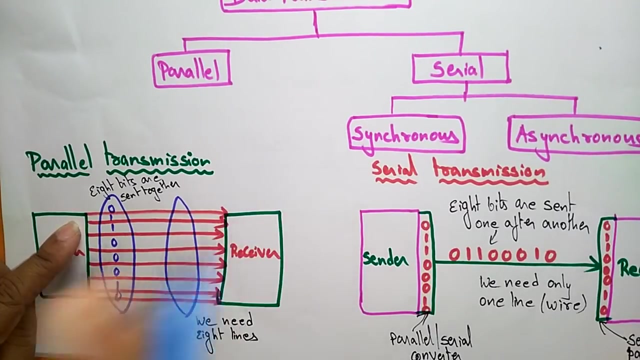 Okay, so the parallel may be synchronous, asynchronous, as well as the serial data may be asynchronous- data you can send, or asynchronous, So you can send. Let's see the parallel transmission. The parallel is nothing, but the sender is there, the receiver is there. If you want to send an 8-bit data, how the data is going to be sent from sender to the receiver. So each bit is single line. This is a 8-bit source sent together At a time. the 8-bits are sending. So that is the main advantage in parallel transmission: At a time you can send the 8-bits on 8 lines parallelly from sender to the receiver. 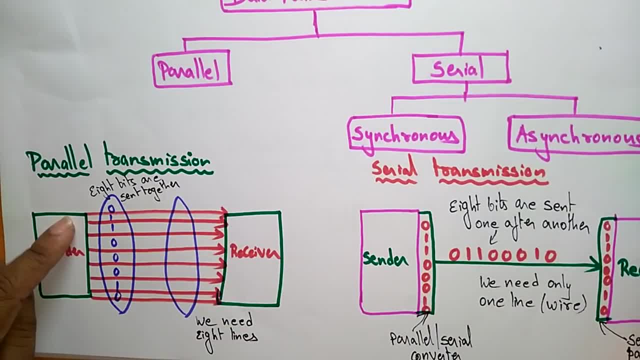 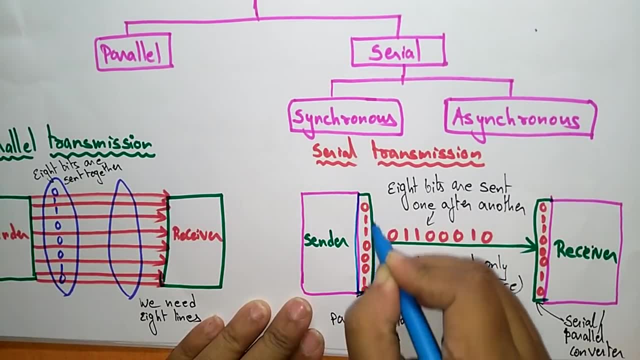 so for that you required eight lines in the parallel transmission. then what is about the serial transmission? the serial transmission? so here you are having the complete bit, eight bit data, even though the center is having the eight bit data here on a single line, one by one. bit is. 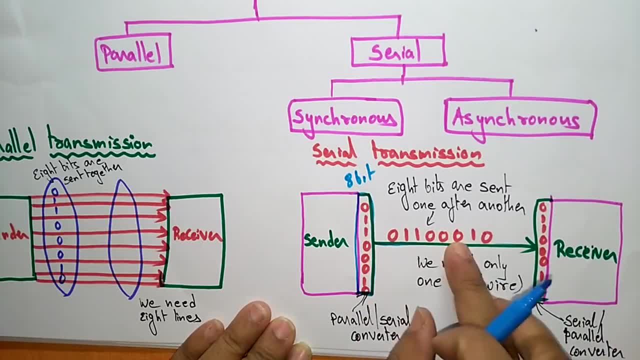 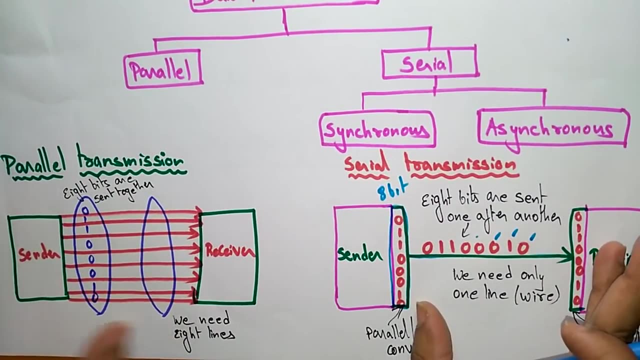 transferred from sender to the receiver. that is a serial. eight bits are sent one after the other: first zero, next one, next zero, like that one after the another. so we need only one line, that is a one wire. that's the main difference between the parallel transmission and the serial transmission. 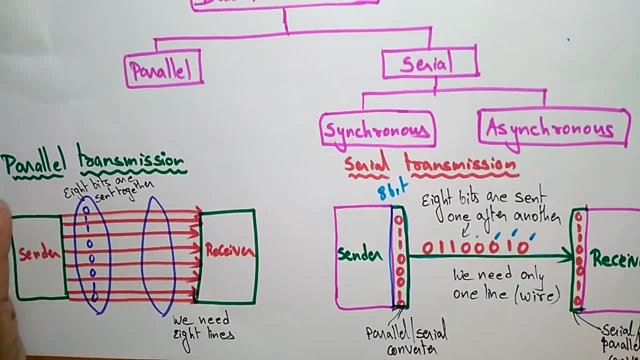 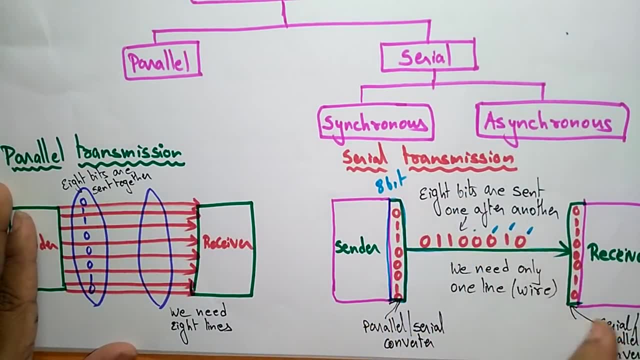 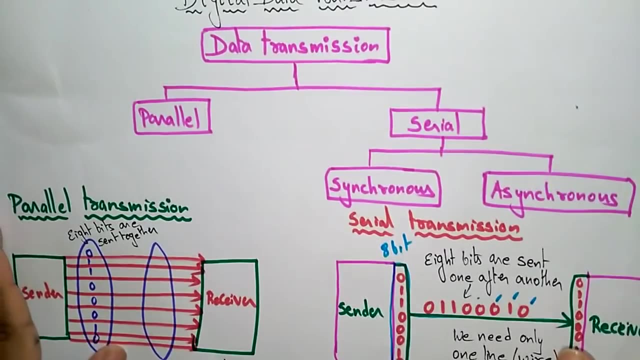 parallel you require more lines, whereas serial you require only one line. so the parallel or see, with the help of parallel or serial converter, you are sending one bit after other so that the receiver can receive the data serially. so this is the difference between the main parallel transmission. 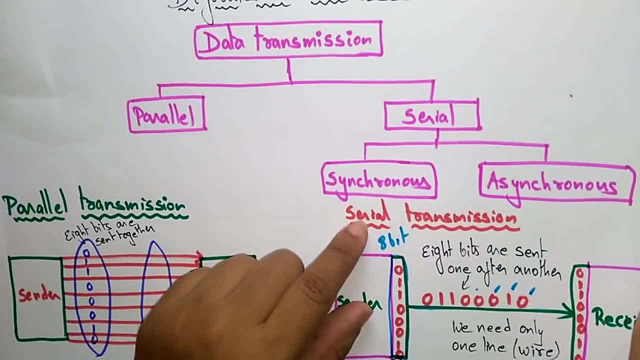 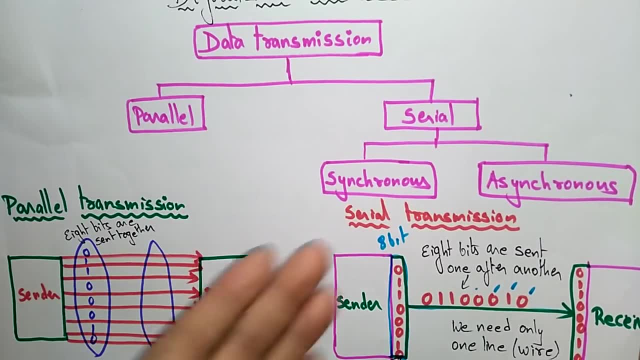 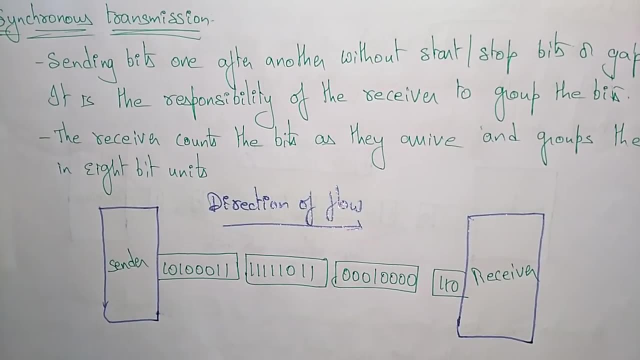 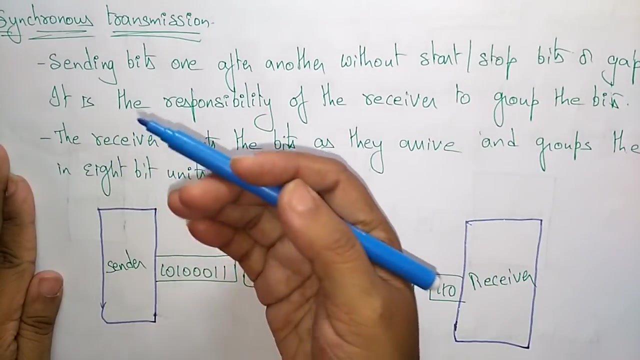 and the serial transmission. so i said it is maybe the data. whatever you are sending, either in a parallel lines or in serial single wire, that may be a synchronous or asynchronous. so what is a synchronous transmission? synchronous transmission, it's nothing but sending bits one after another without start or stop bits. so we are talking about this serial, uh, in the serial transmission. 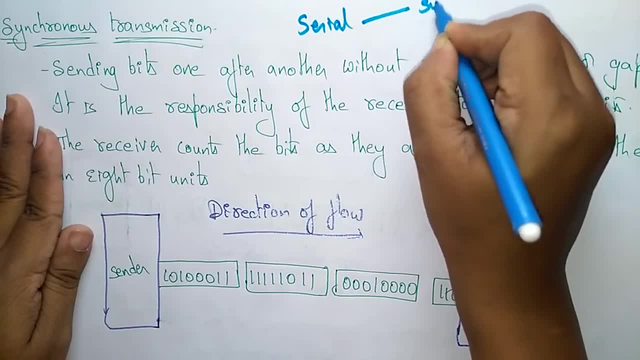 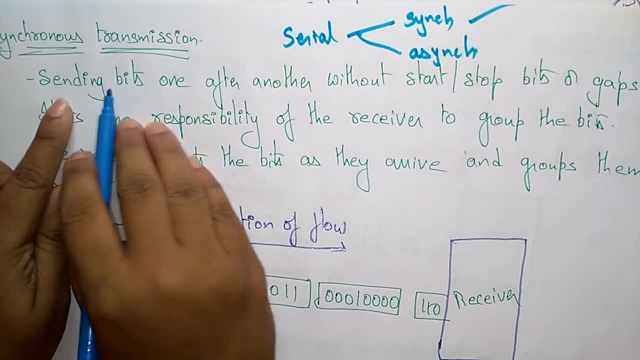 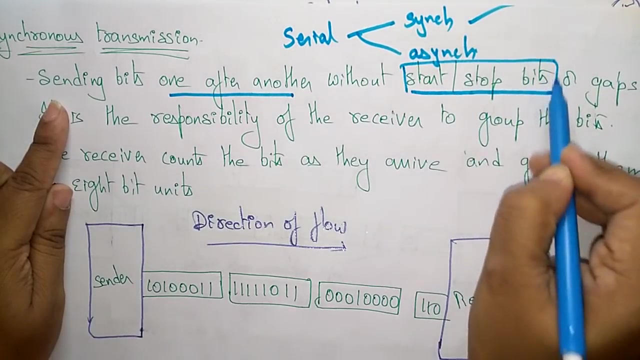 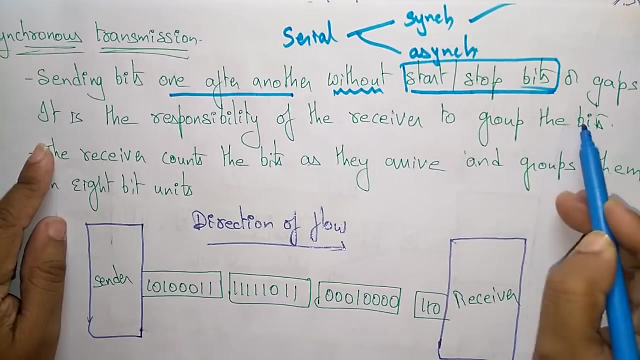 the serial data may be asynchronous or you can send asynchronous data. so what is synchronous? synchronous means sending bits one after another without start or stop bits. so without without start or stop bits or gaps. it is the responsibility of the receiver to group the bits. the main responsibility of the receiver is to whatever the data, that is, the sender, is sending. 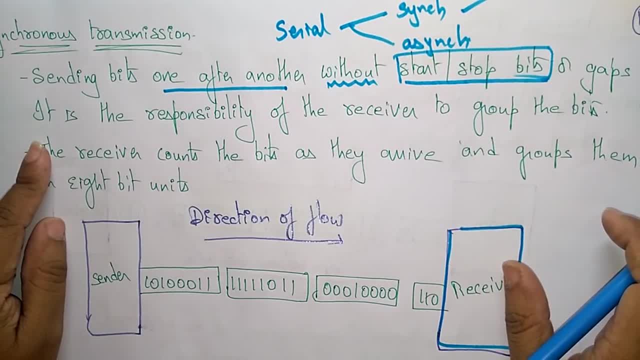 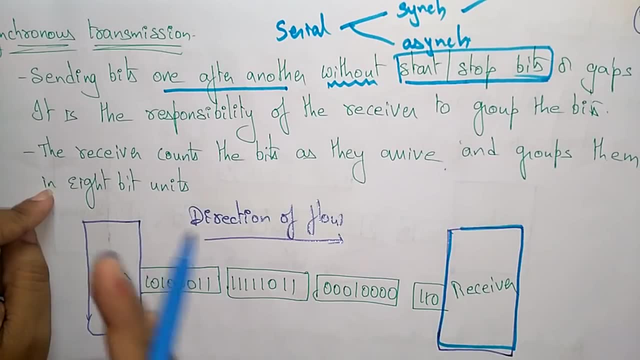 that has to be arranged accordingly. he was your wish. so the receiver counts the bits as they arrive and groups them in 8-bit unit. so the receiver is going to be counted one, next, two, next, until whenever he receives 8 bits. okay, one byte of data i received, so next he takes another. 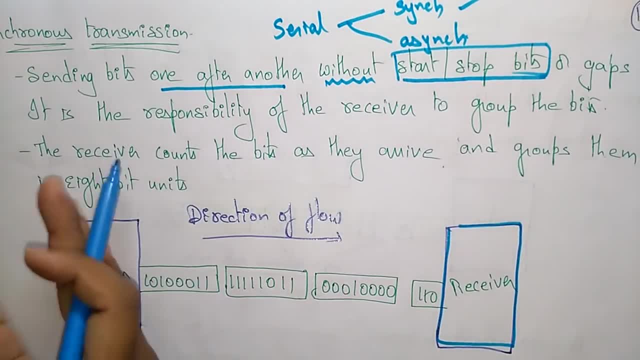 like that. the receiver's responsibility is he has to check here. the sender is sending bits one after another without start or stop bits. so the receiver is going to. sender is sending the bits. okay, here 8 bits are sending. okay, the receiver is going to receive one. 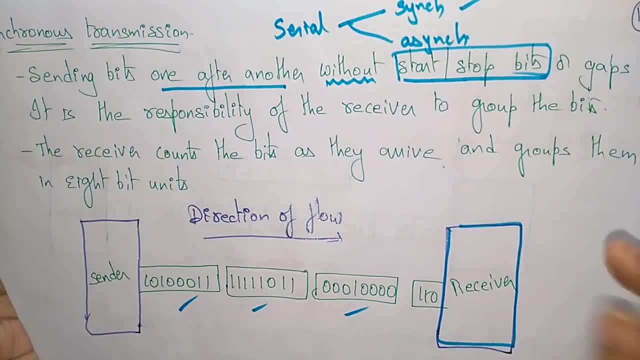 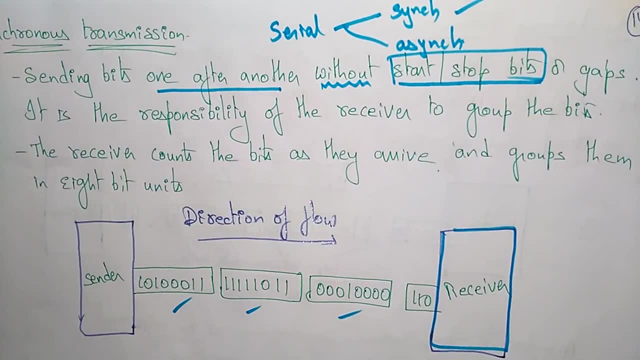 bit after another. okay, whenever the 8 bits are completed, okay, one byte of data is received, like that, the receiver responsibility. so, in the same way, whatever i am recording the videos, i am sending the videos one after the another and i am uploading in the youtube. okay, it's your responsibility, your. 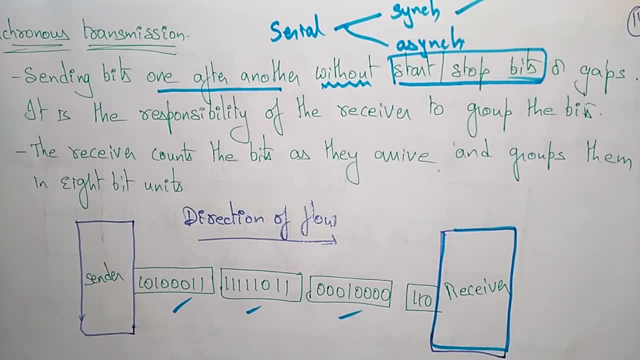 receiver. so what is the next sequence of this video? so this video after the continuation is: what is the next video and what is the next video? you have to group that and you have to make one subject like that, okay. so this is a synchronous transmission. so whatever i sending and whatever you are receiving, 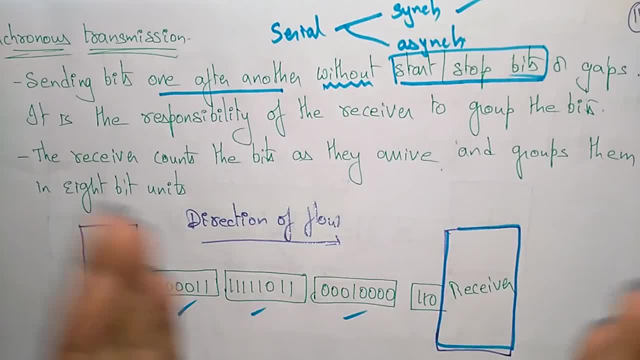 is a synchronous transmission whenever the suppose one topic is divided into three videos. so whenever the three videos are over, that topic is completed. so the receiver, you, you are the receiver. you decided: okay, the three videos are completed and one topic is, uh, completed like that. then what about the asynchronous transmission? asynchronous transmission means: 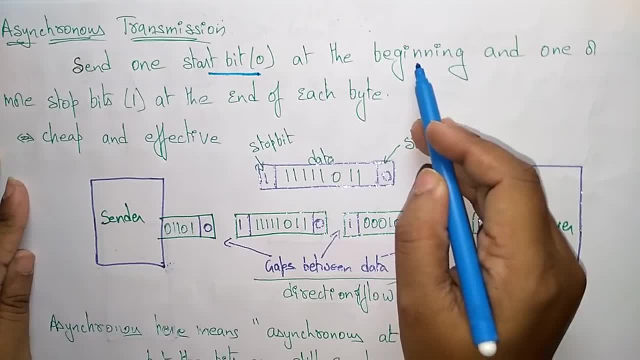 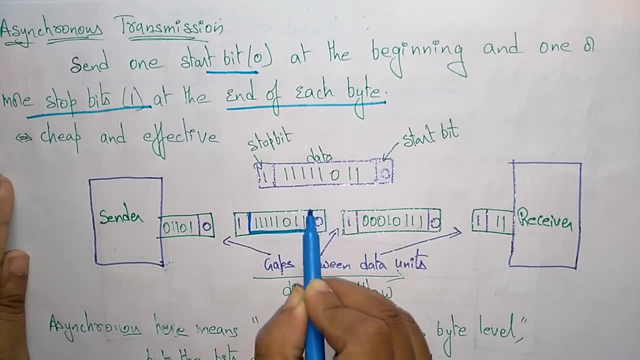 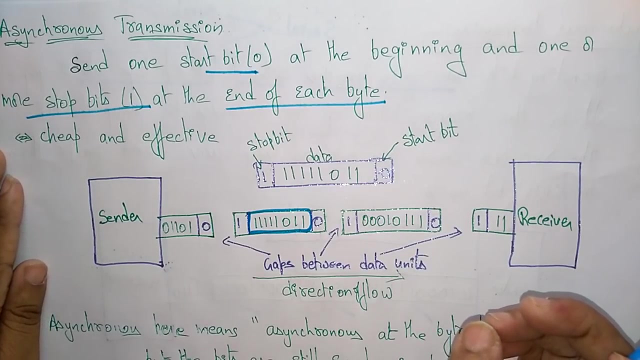 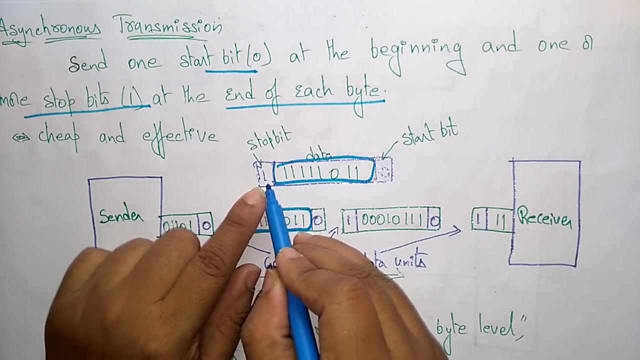 send one start bit, zero at the beginning and one or more stop bits at the end of each byte. so, whatever the byte information, is there eight bits. so starting and ending, send one, uh, one start bit and zero or one stop bits. so here see, this is eight bit data, one indicates stop bit. 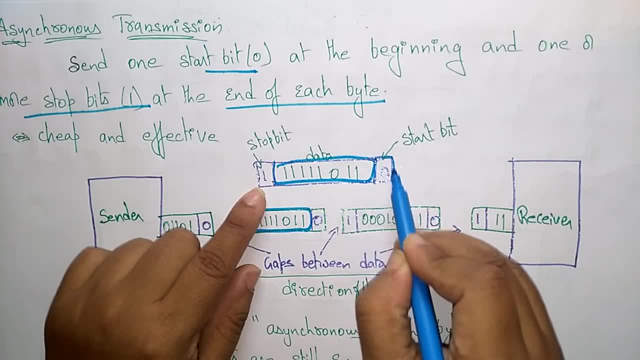 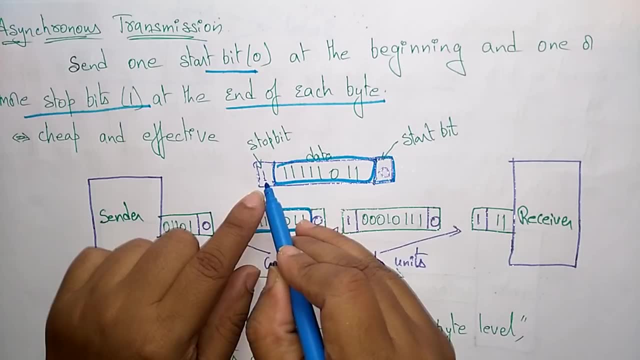 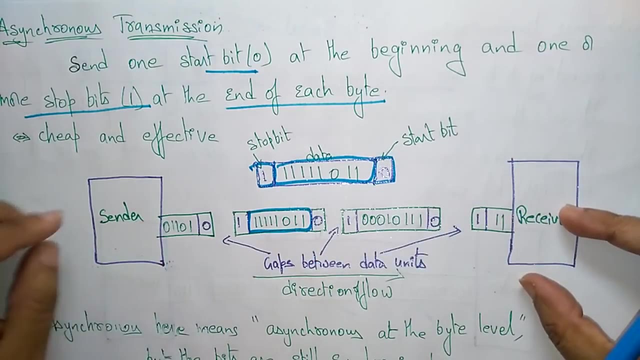 zero is start bit. so whenever the receiver sees zero, the next information: whatever he is receiving: eight bits okay. after that, whenever he sees one, okay, this data is completed. next data is coming. so with the help of start and stop bit, the receiver can understand the complete byte of data. 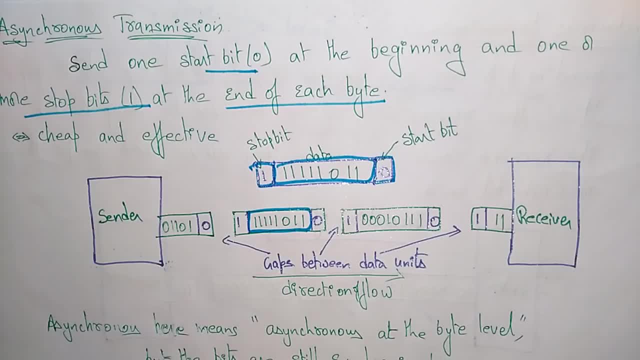 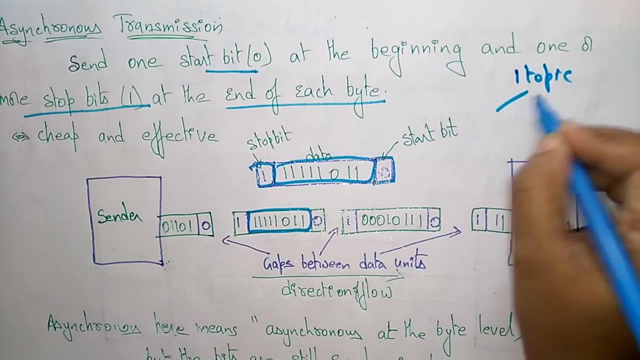 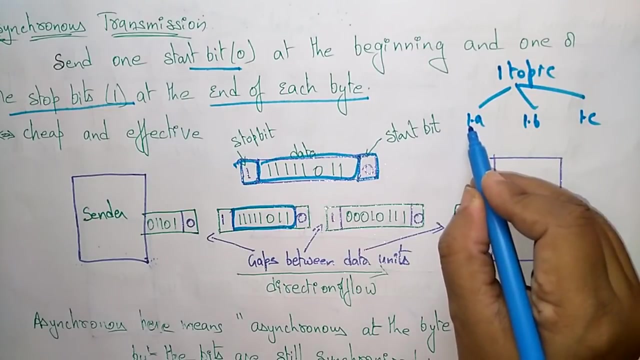 it is this: asynchronous transmission is cheap and effective. let's take my videos, okay. so if i send uh, if i mark the videos, if i give the numbering to my video, okay, suppose, uh, one topic i divided into three videos, okay, so one a, one b, one c. so whenever you have seen one a, one b, one c, your, you thought 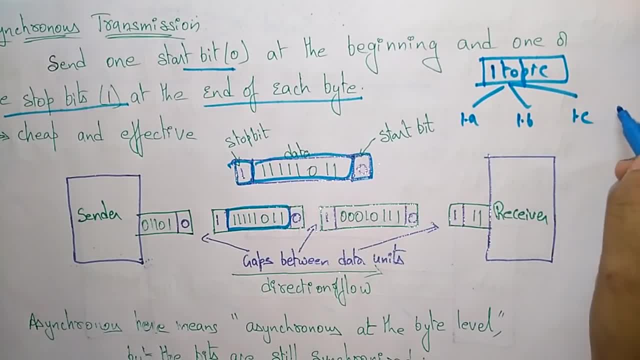 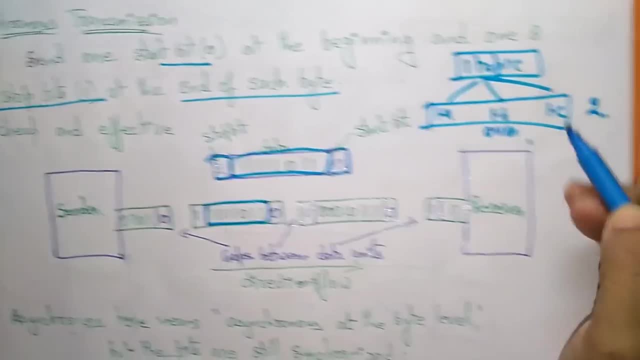 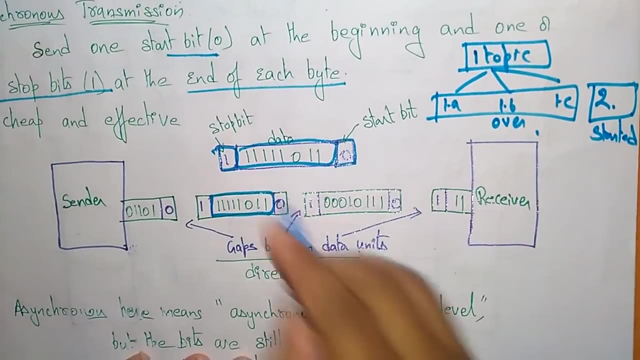 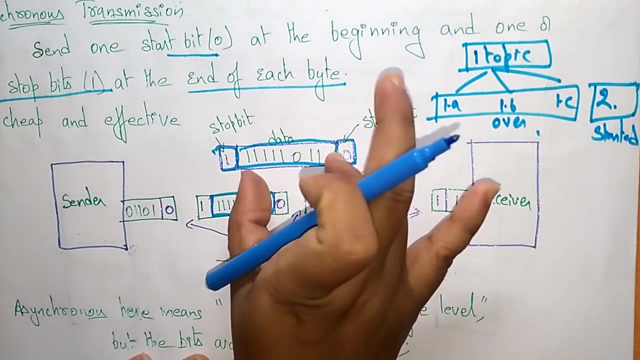 that it is completely related to this topic. so whenever the next video is two, it indicates two. you will understand this topic is over. next second topic is started. so that is a start and stop it. it's indication. the receiver is indication with zero, and one zero means start bit. so after zero it takes eight bits. 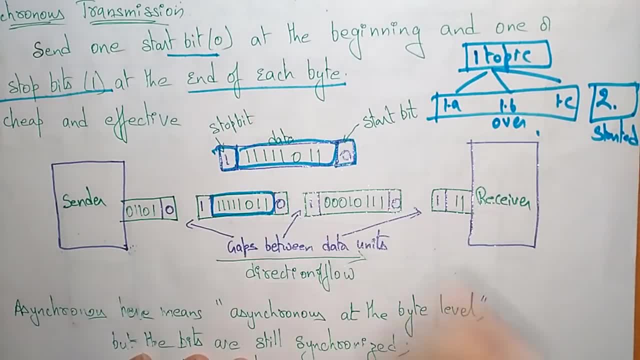 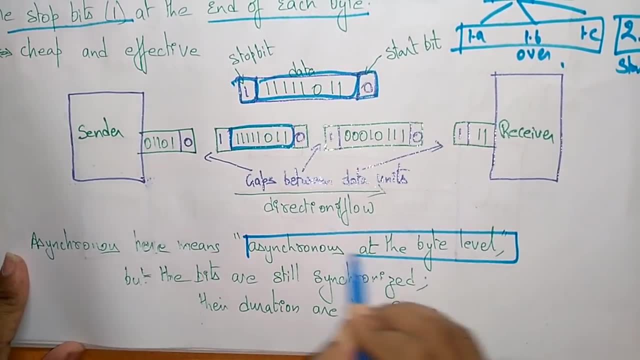 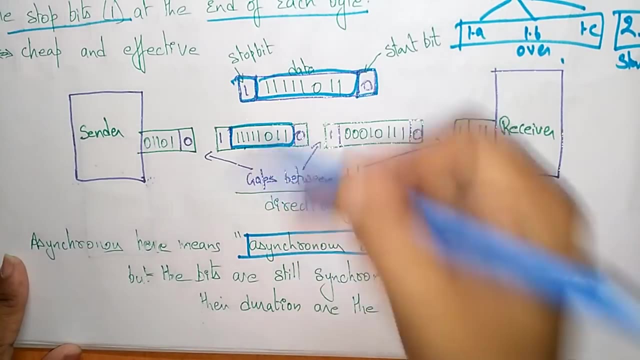 after whenever it receives one. okay, this data is over one. stop it. asynchronous here means asynchronous at byte level. you have to remember this. asynchronous at the byte level this data is: click abused password changes. that literally opens. and now the diagram, the chart. academics has maintained that the same age decision decades goes on. and as the data is,